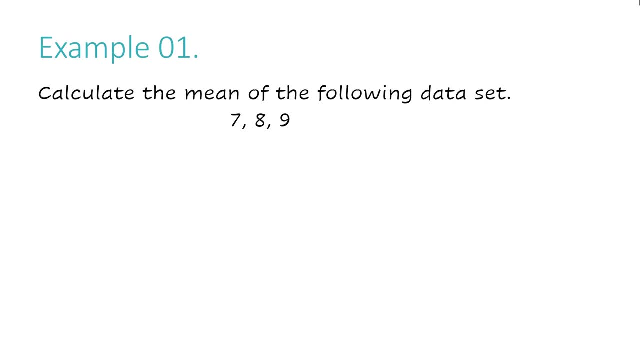 Example number one says: calculate the mean of the following data set: My numbers are 7,, 8, and 9.. If I were to add these together- 7 plus 8 plus 9,, I would get 24.. If you remember when I explained, 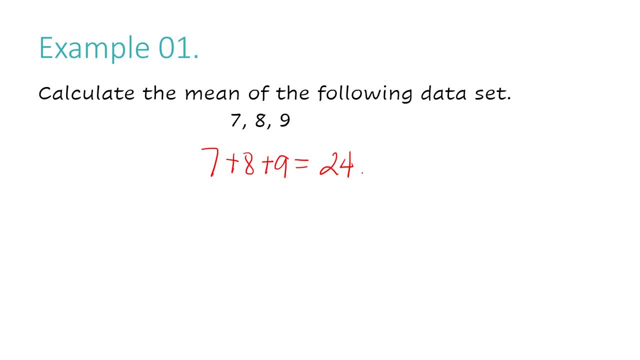 how to calculate mean. I said you need to divide the sum of the numbers in your data set by the number of values that you have. So if I were to add these together I would get 24.. Example number two says: calculate the total amount of numbers in your data set. 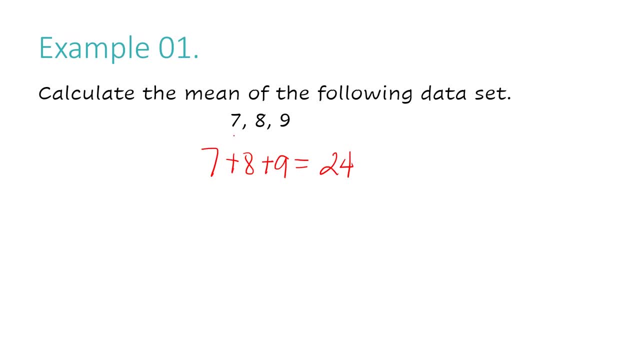 So the total amount of numbers in my data set is 3, because I have 1,, 2, 3 numbers. So I'm going to take my 24 and I'm going to divide it by 3 and I'm going to get 8.. 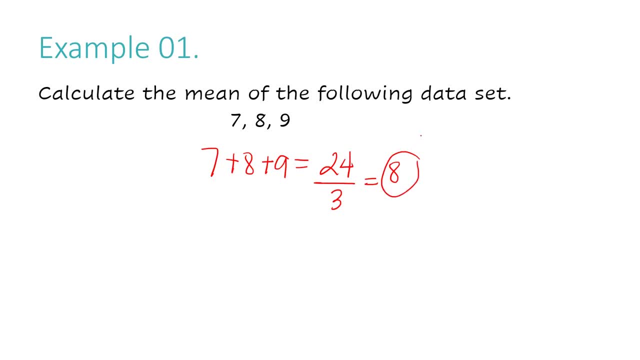 So the mean of the data set 7,, 8, and 9 is 8.. Let's take a look at example number two. Example number two: Calculate the mean of the following data set. Well, again, I'm going to start by adding all my numbers. I have 4 plus 5 plus 3, plus 9, plus 8 plus 12 and plus 1.. 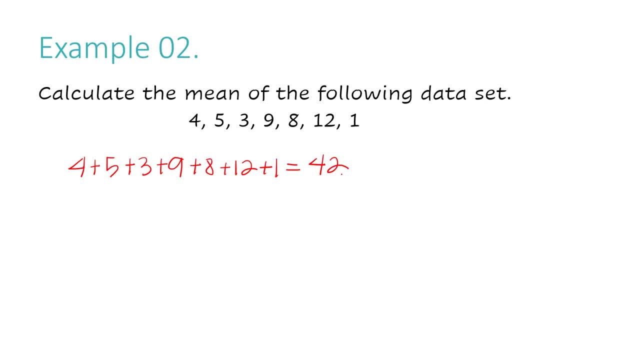 And that gives me a total of 42. Then I need to divide 42 by the total number of numbers in my data set. Well, I have 1,, 2,, 3,, 4,, 5,, 6, 7 numbers. 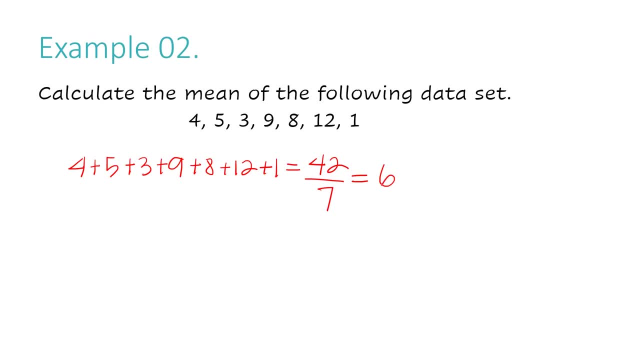 So I have 42 divided by 7, and that gives me 6.. And, by the way, 6 times 7 equals 42 is my favorite multiplication fact. Anyway, let's move on to example number three. Example number three: Calculate the mean value of even numbers from 65 to 78.. 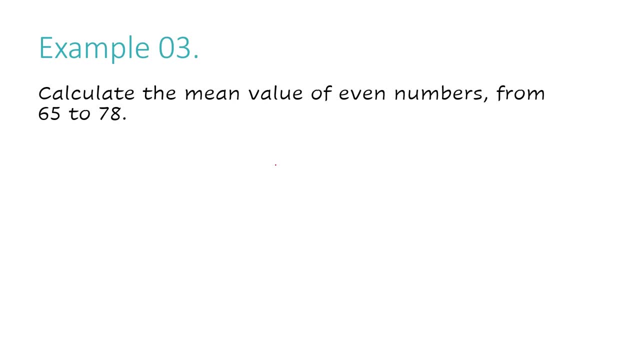 Well, this one's a little more complicated because they didn't just give us our data set, So they want us to find the even number. So we're not going to use 65.. We're going to use the next number after 65, which is 66.. 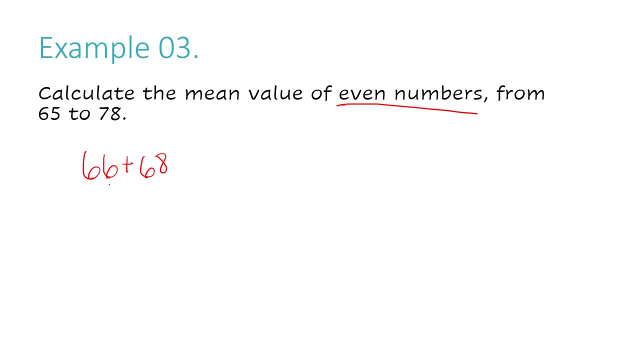 66 plus 68. We got to skip 67 because 67 would be odd right. So 66,, 68,, 70,, 72,, 74,, 76, and 78. When you add all of those together you get 504.. 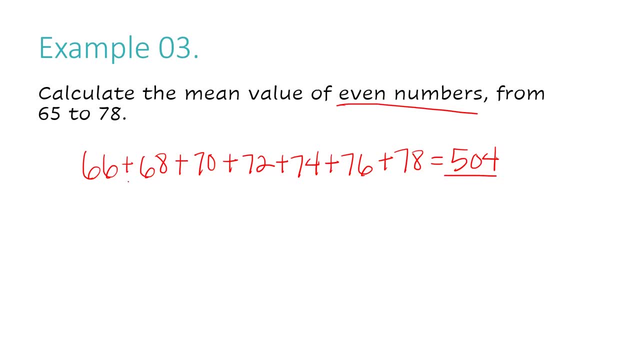 Now I need to divide 504 by how many numbers are in my data set. Well, I got 1,, 2,, 3,, 4,, 5, 6, 7 numbers. So that's 504 divided by 7, and that gives me 72.. 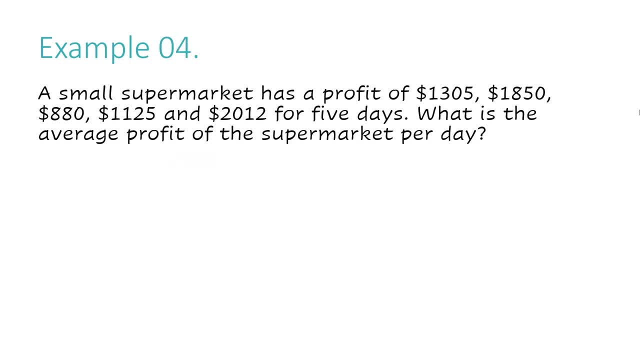 Now let's move on to example number four. Example number four: A small supermarket has a profit of $1,305.. $1,850,, $880,, $1,125, and $2,012 for five days. What is the average profit of this supermarket per day? 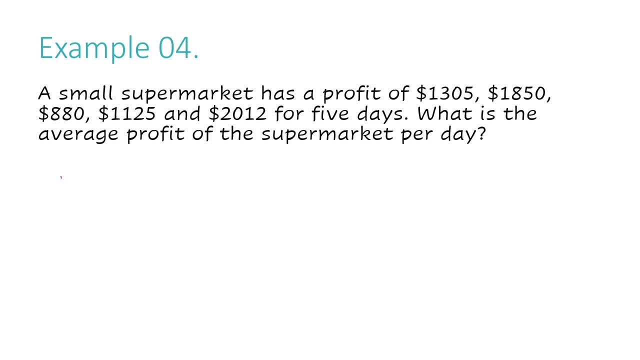 So we're going to add up our amounts. We got $1,305 plus $1,850 plus $880 plus $1,125 plus $850.. That's $1,212.. When I total those I get $7,172. 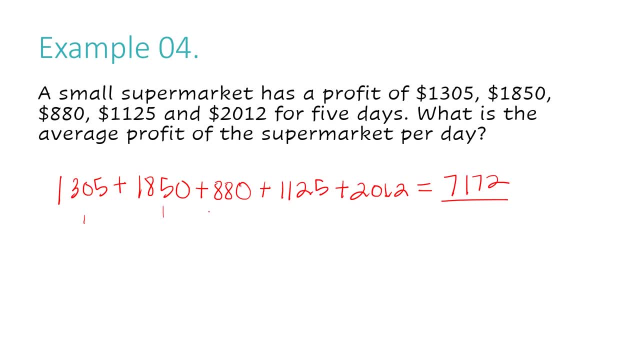 Now I have to divide by how many numbers I have. I have one, two, three, four, five numbers. Now I take 7,172 divided by five and I get 1,434 and four. If you were to type that in, you would get $4,144. 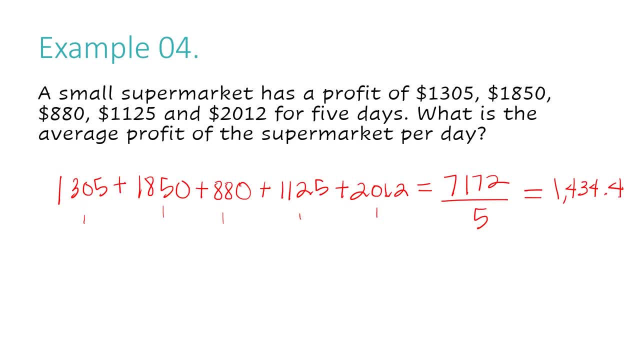 $4,144.. $4,144.. the calculator: you get one thousand four hundred thirty four and four tenths. well, because this is a dollar amount, you're gonna add a zero so that you can complete your change. you wouldn't go to a store and it's not. it's not gonna give. 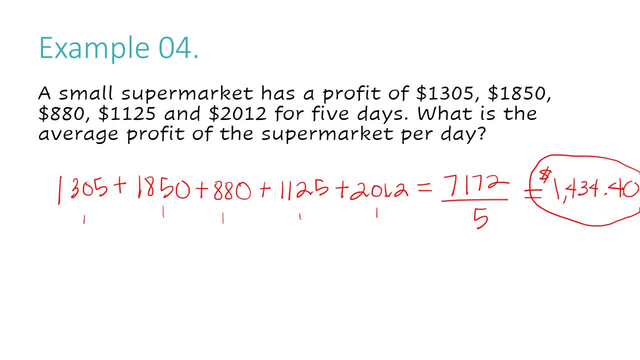 you a dollar amount, point one digit, it's gonna give you two digits. if you're dealing with, like US dollars- some other countries may show their money a little differently- but for the United States- and you're talking about regular dollars- it's gonna be decimal in two digits, not just one digit. so you need to add a zero. 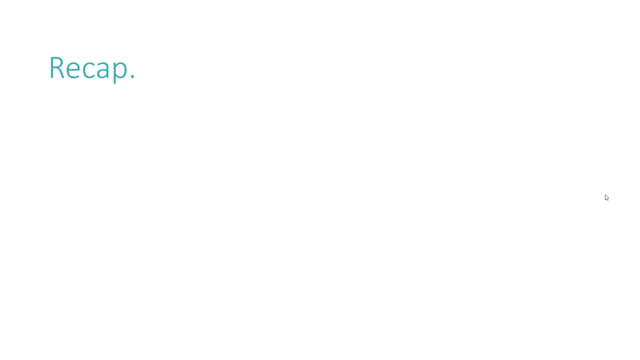 now let's take a recap. here's our recap. first, add up all the values to find their sum, then count how many numbers are in the data set. finally, you're gonna divide the sum of all values by the number of values. now you try. I want you.